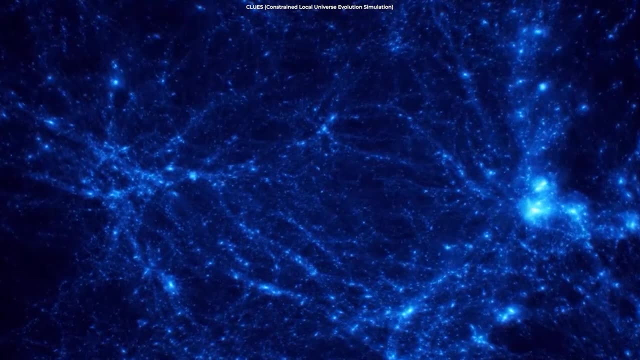 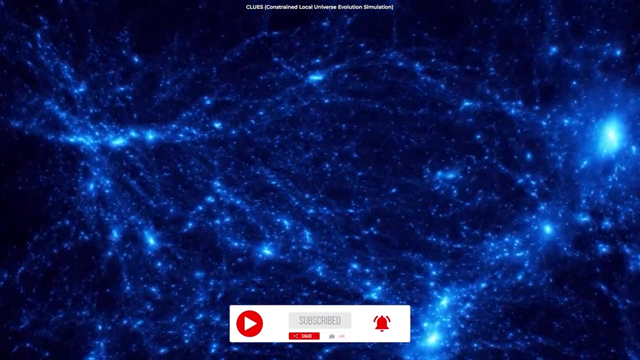 These filaments are the largest structures in the universe, stretching hundreds of millions of light-years in length and about 20 million light-years in thickness. Not only are they home to millions of galaxies, but contain most of the universe's mass. Cosmic filaments are separated. 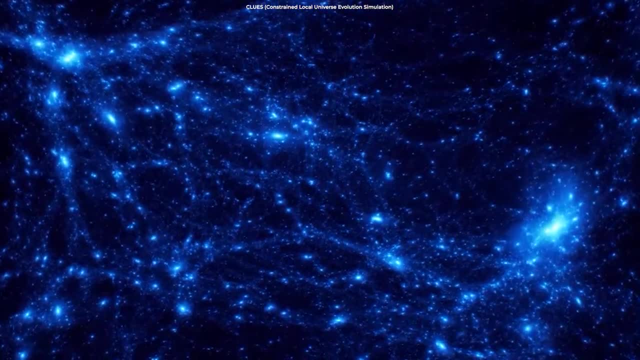 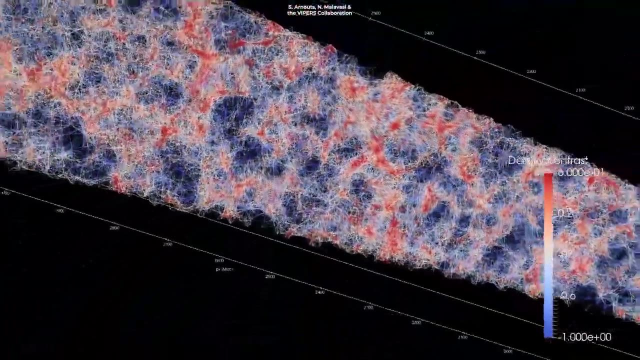 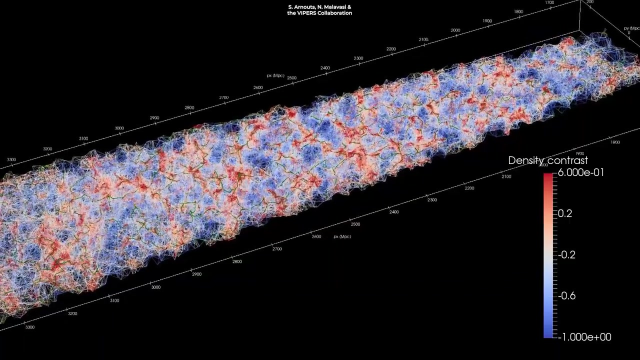 by huge cosmic voids, which are relatively emptier, meaning they contain very few galaxies compared to the strands. The combination of these interconnected filaments, separated by voids, creates what's called the cosmic web, a term coined in 1996 by astrophysicist Richard Bond. 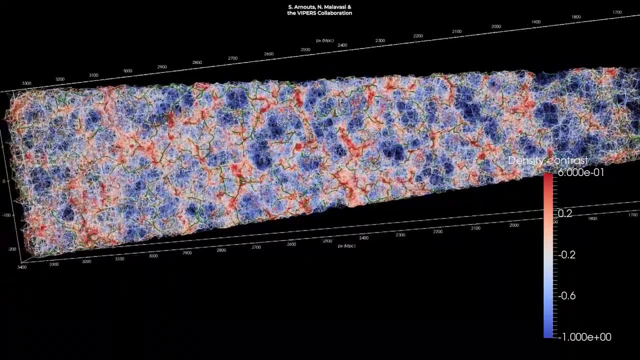 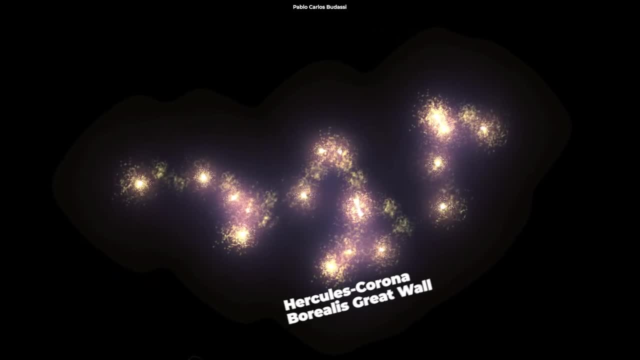 to describe a tangled structure of clumps and filaments created by dark matter. The largest known filamentary structure is the Hercules-Corona-Borealis Great Wall. This beast is 10 billion light-years long and is home to several billion galaxies. 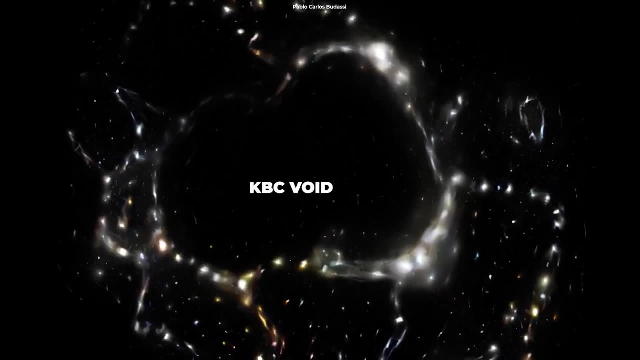 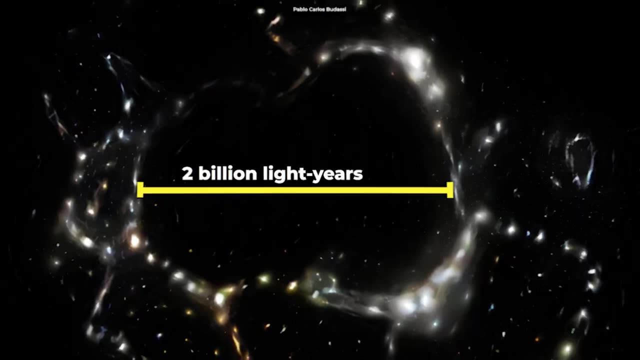 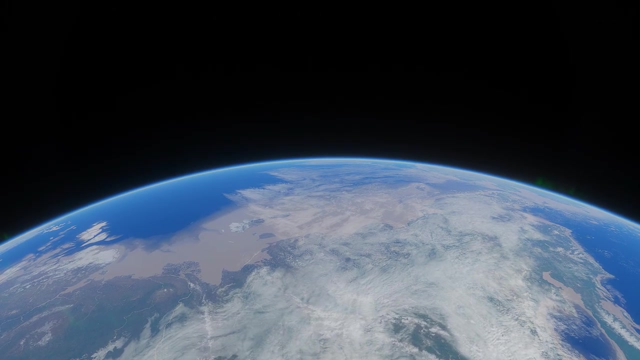 On the other hand, the largest void is the KBC Void, short for Kenan, Barger and Cowie. This loneliness has a diameter of 2 billion light-years. You would think that if we were part of such a void, our night sky would be truly dark. Well, let me tell you. 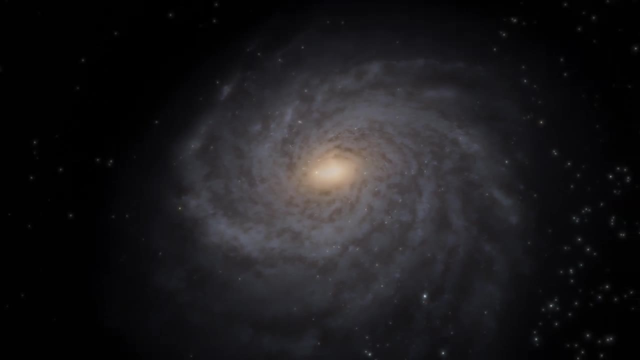 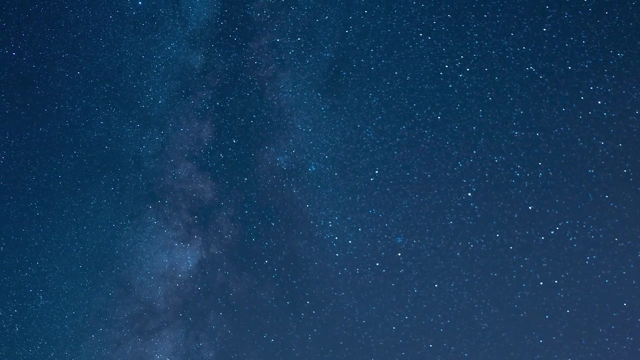 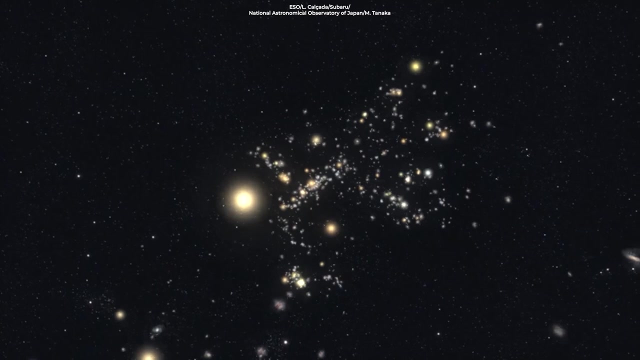 the mind-boggling story. Our own Milky Way is part of the KBC Void. We are part of the biggest void in the universe, yet our night sky is full of light pixels. Whether we're part of a filament or a void, it doesn't matter to us, because we are puny compared to the vastness We can't tell. 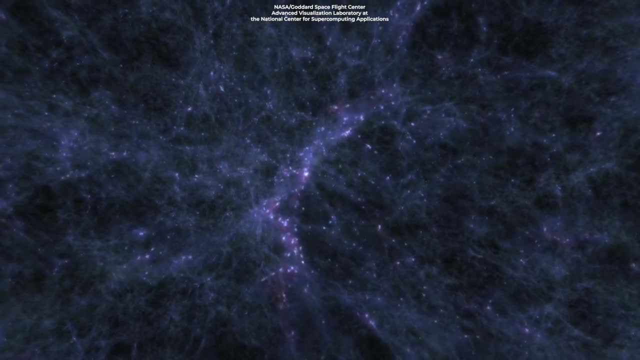 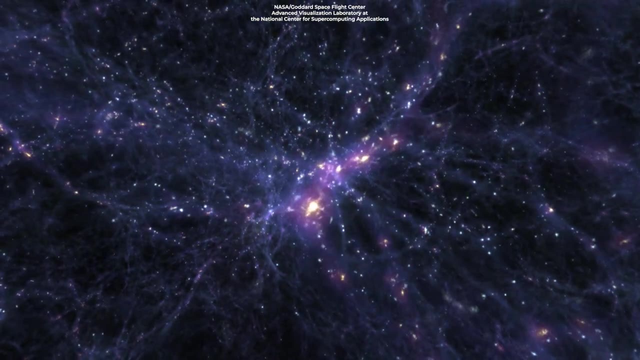 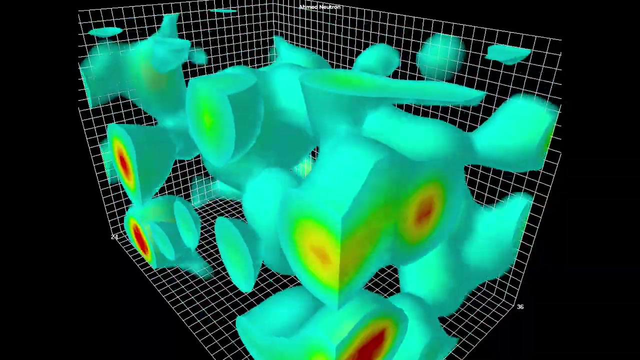 the difference. Theory suggests these super-vast structures are formed by what's called hierarchal clustering, which is the process by which larger structures form through the continuous merging of smaller structures. This means galaxies gathered around primordial density fluctuations, which are quantum mechanical fluctuations in the density of the universe. 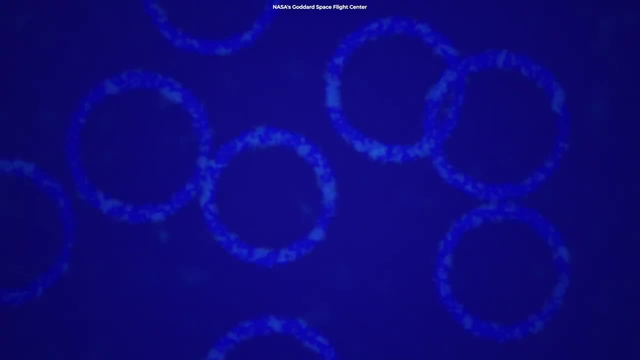 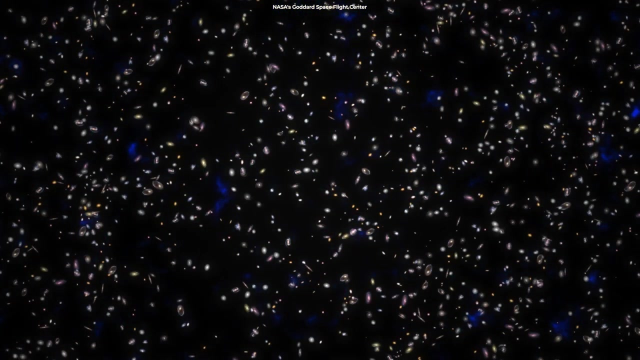 in the very first moments after the Big Bang. As the universe expanded, those fluctuations got bigger and bigger and the universe turned into regions of higher and lower densities of matter. thus the filaments and voids- Cosmic voids- make up most of our universe. 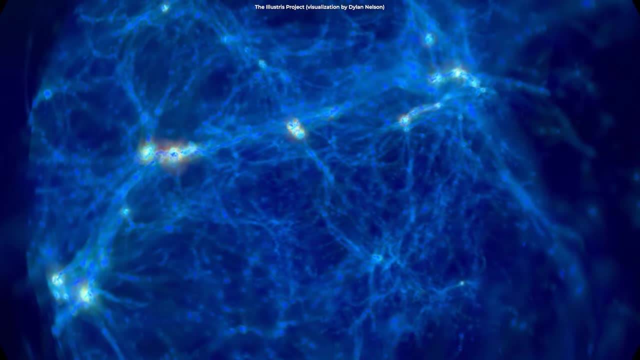 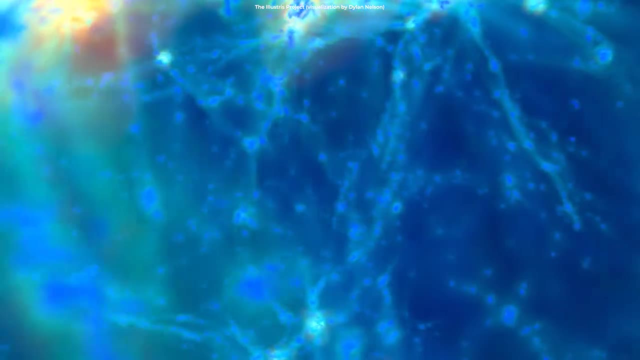 and, based on recent studies, we can say that the universe is a very large universe. Based on recent studies, they may be the reason why the universe is expanding at an ever-accelerating rate. That's because, according to a paper that we linked below, cosmic voids may be the source of